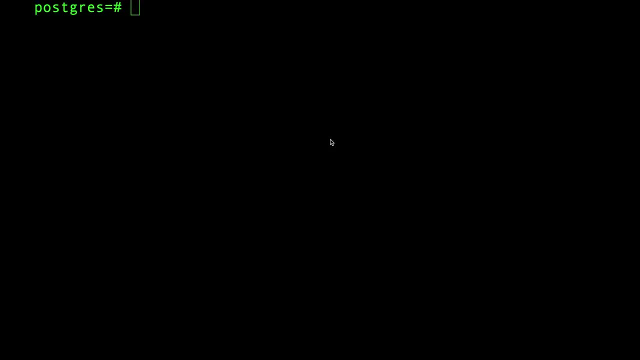 So, first of all, what is an index? An index is is a data structure that you build and you assign on top of an existing table. that basically it looks through your table and then tries to analyze it and summarize it so that it it can create kind of shortcuts The the best way I 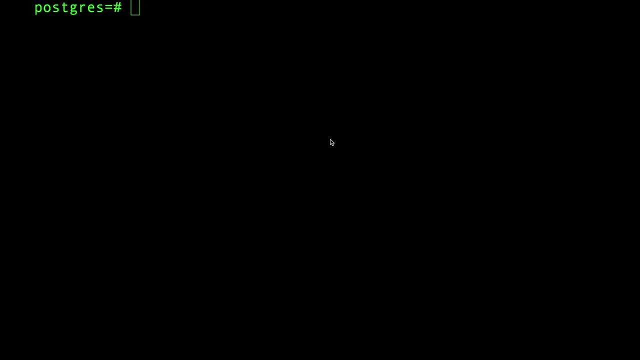 can think of indexing is really by considering 15 nào cleaning data together and American application beta and fácil analysis basic table so that fast, under any conditions, and then we have it on a business indexes like if you know these, uh uh, if you have, if you ever seen a secretary's uh uh handbook or 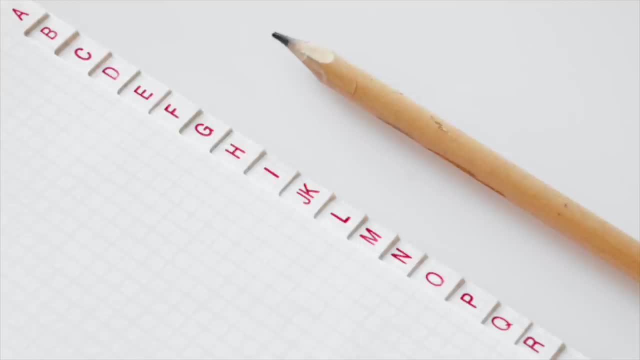 phone book where you have like thick big book and it is labeled. there's like a label color with a, b, c, d until z, right. so the the the letter a starts with all the company's phone books. that, uh, that start with the letter a and b start with all the b's right and c is all the c. so if you want to, 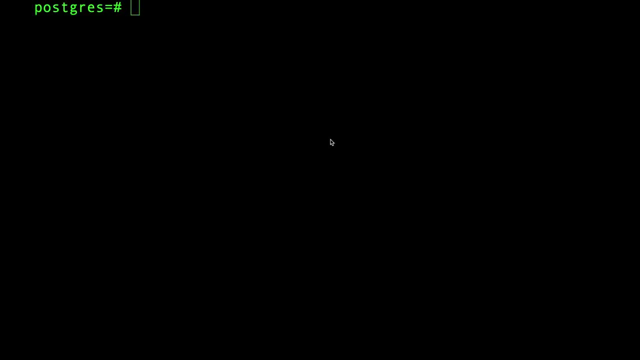 look through, uh, find a specific company name, phone number, and you know it's like: oh, it's, it's i don't know, it's called zebra. so you go immediately, you go to the z right and then you start searching there. it's, that's the simplest thing i can think of the index right and, uh, basically the index guys. 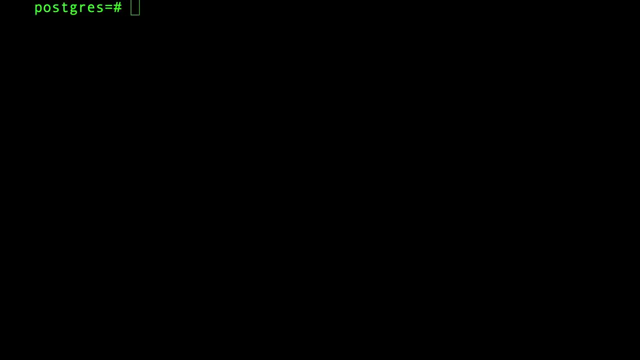 are are are two types so far that we know of, uh, something called b3 and lsm trees, and i'm not going to go through that. you the depth of how they are constructed. this is outside the scope of this video, but essentially it's a, it's a data structure and you can look it up. it's basically allowing you to search very. 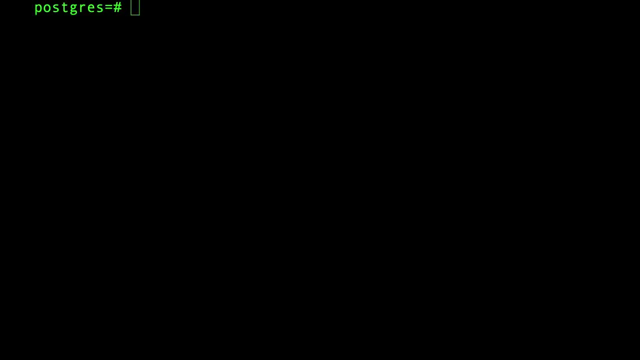 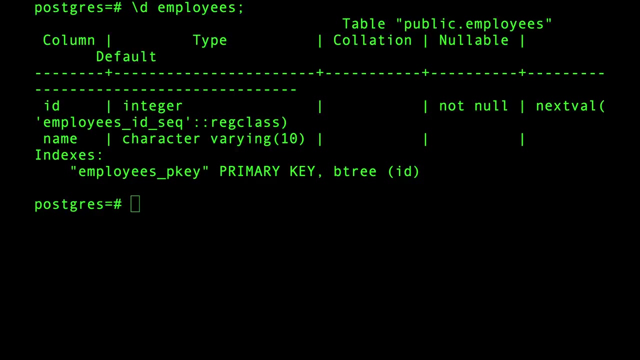 effectively right and, uh, you find quickly what you're looking for. so, guys, here i have a table called employees with around 11 million uh rows. okay, it's a quite large table. okay, so i have an id field is integer, it's not null and it's sequential, so every time i insert a row, 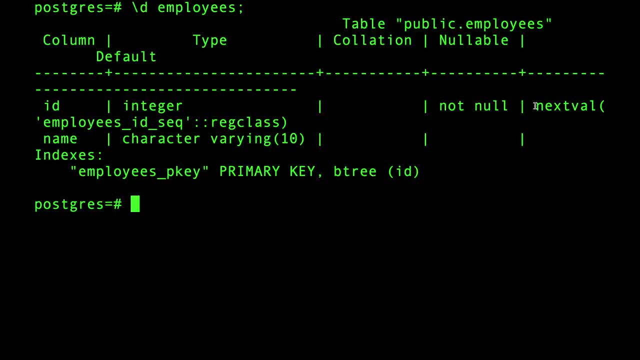 i don't touch this field. it will automatically insert and increment the value and it's also a primary key. that means unique right and it also has an index by default. every primary key has an index by default and it's a b3 index right. so that's what i have here. 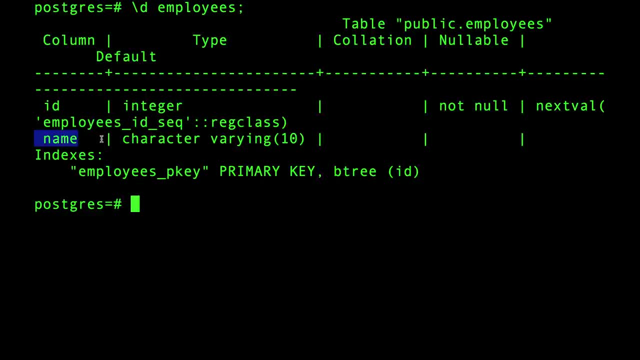 and i also have a name field on this, which is what? doesn't have an index. it's just a bunch of characters, nothing fancy. it's not really the actual name. i just spent some time generating 100 million random strings, right? so so now if i, for example, do- uh, let's clear this up and do select. 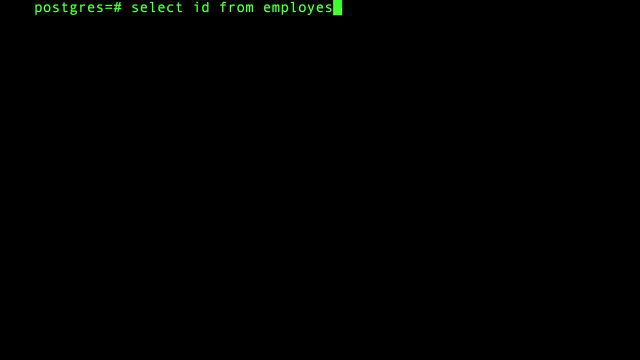 id from employees. uh, where id equal thousand, i will return the thousands id, right? that's? that's not fancy, right? so if i do select star, i will get everything back: id and name, and nn1 is the name, so so don't don't pay attention to the actual name, it's just. 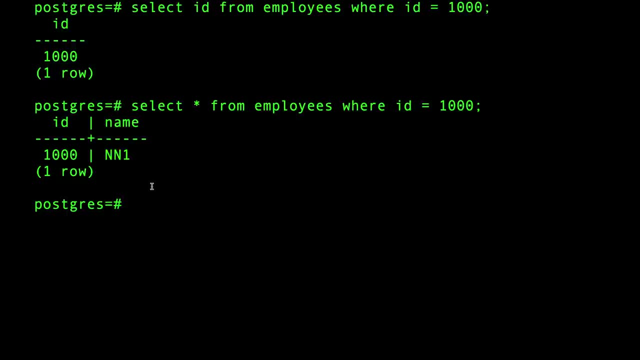 a string, and that's the idea of the string here. so, guys, what i want to do here is i'm going to go through steps of different queries. i'm going to show you the performance of each of these queries, right in order to do that in postgres- that's the database i'm using- i'm going to go through. 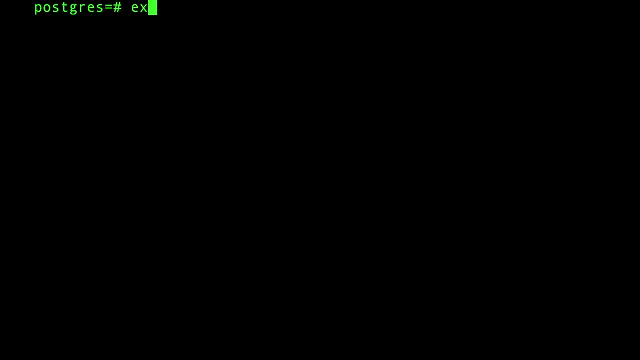 postgres, i'm going to do explain analyze, which will actually explain the query that i'm going to do, and it's going to tell me how long it took, right, which is which is really neat. so i'm going to do select id from employees where id equal, let's say 2000, because the first one is cached. 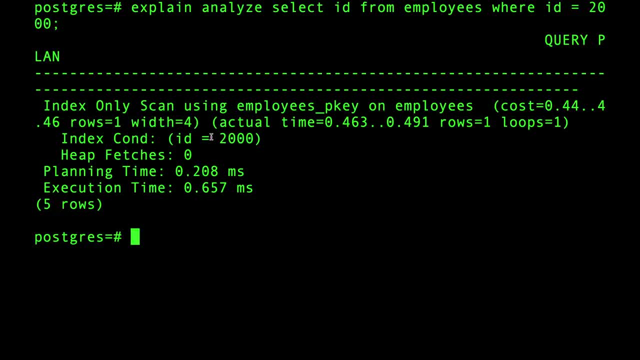 i don't want to mess up the statistics, all right, so what happened here, guys? let's let's decipher what happened. it says: okay, your predicate filter, you're trying to find id 2000, that's the employee with id 2000. you know, in order i, in order to find that i didn't go through the actual table, 11 million. 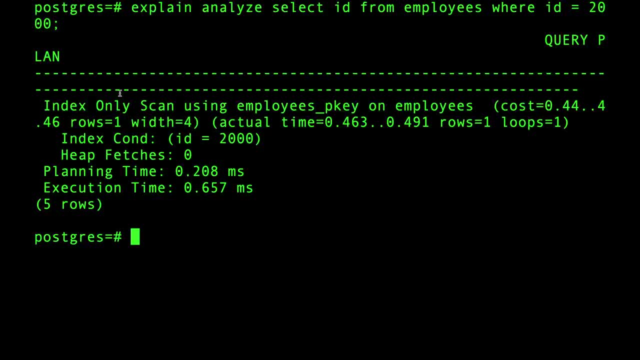 and i searched sequentially. no, i actually scanned the index, which is way faster, because the index is always smaller than the actual table, because it tells you: okay, it is structured in a way so that if you search- and i'm going to put an animation here a little bit- 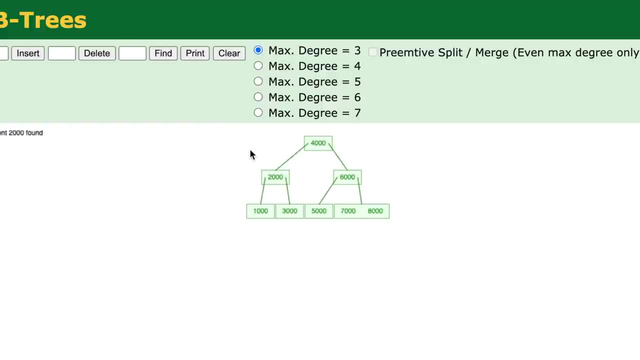 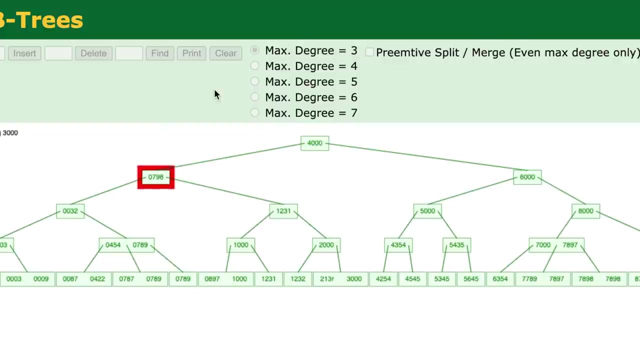 you can see like if i want to find id number 2000, it starts searching. okay, 2000 is between four thousand and and one thousand. so it was okay, let me go to this tree. so it goes. you go to the another tree and then search for from another between this number and this number. so until you, 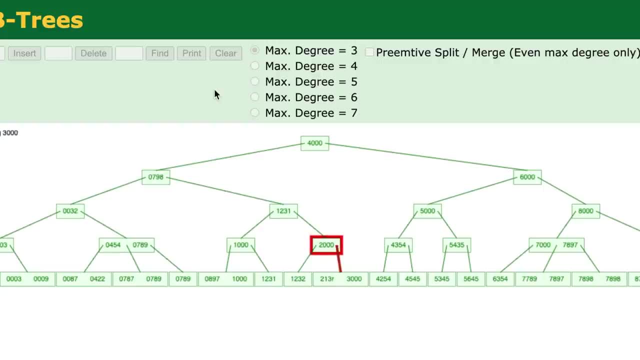 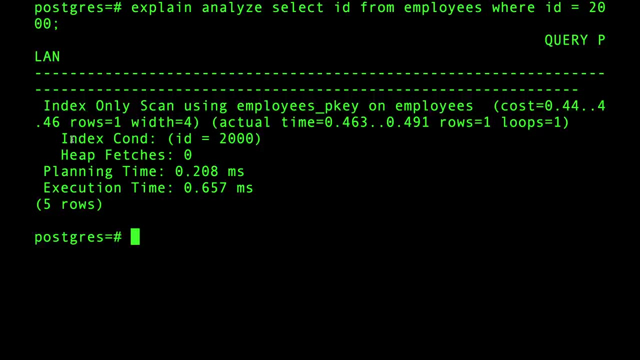 actually find the number right. that's how b3s basically work, right. so now what i did i? i only scanned the index, which is very, very effective, right, heap fetches. that's another uh interesting thing. so says the value that i actually queried, which is the id. i did not have to go to the heap. 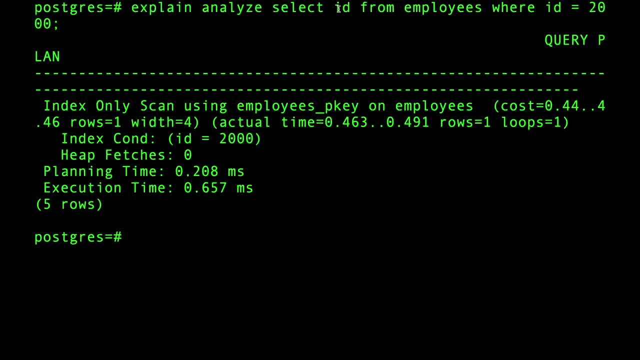 to fetch this information because the id- since that's the only thing you're selecting- is in the index, so i just pulled it in line. that's called inline query, if the information is available in the index. that is the sweetest query to a database in java, so i just pulled it in line. 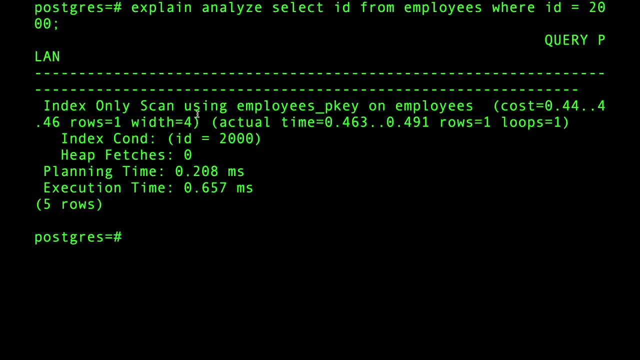 here. if you can put as much information as you can in the index so that, as i, as i scan the index and you only select the id, that is the sweetest thing you can do. so the whole thing took 0.6 millisecond and uh, to plan the query and and to to study what we go through: the i the the fact of 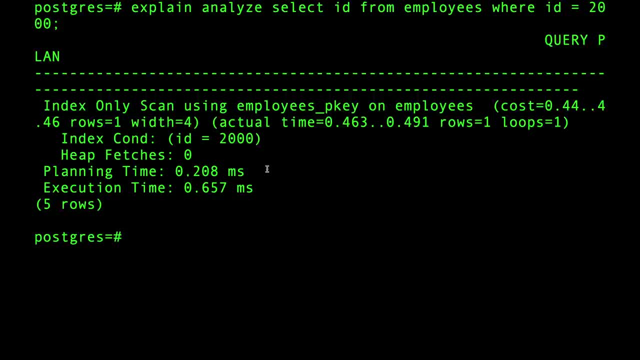 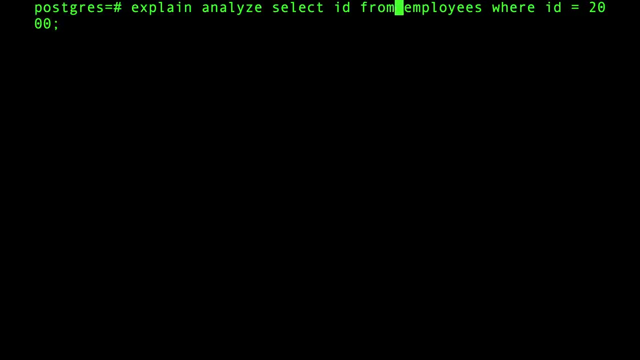 oh, should we use the index or should you scan the table? is a query, is a decision and that's called the planning time. execution is the actual work. to go and do the work, all right, so let's spice things a little bit. what i want to do here in this case, i want to uh. i want to select uh 3000 in this case. 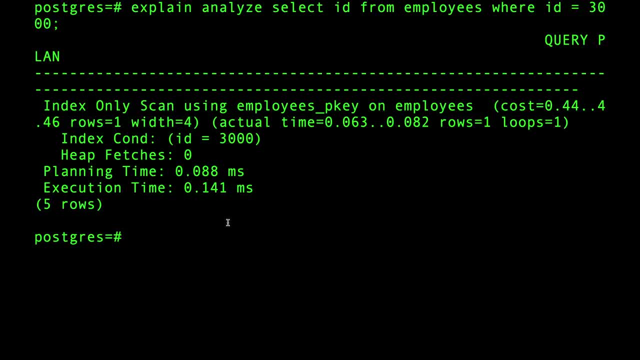 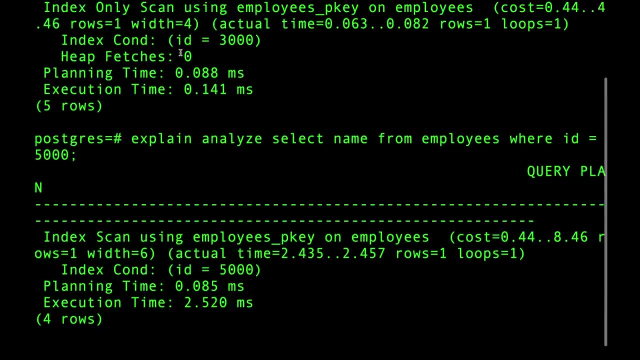 and you can see that took 0.1.8. what i want to do is i'm going to change the id 5000 and instead this time i'm going to ask for the name and compare the the that cost here. guys. look how long it took. So selecting only. 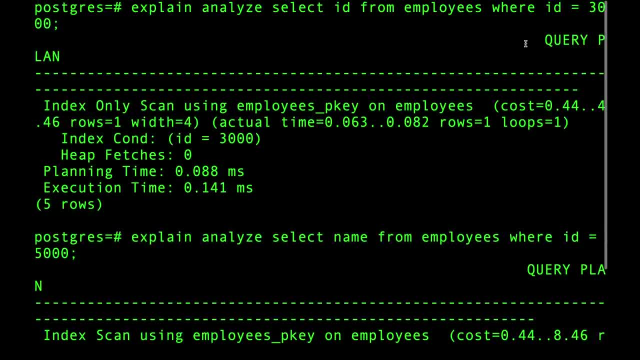 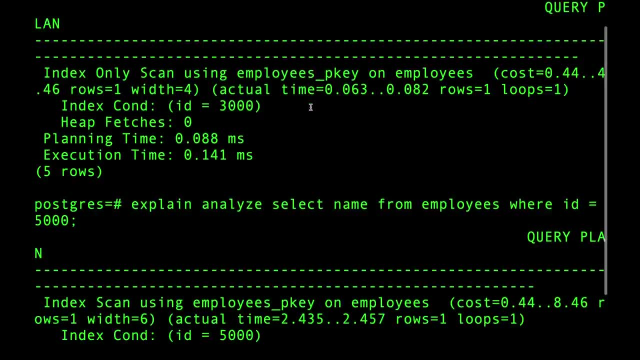 the ID, where you know the ID, which is like a silly query, if you ask me. right, it's a little bit of silly query because you know the ID. why are you just selecting ID? but it's just for science, guys. we're doing this for science, So it's pretty. 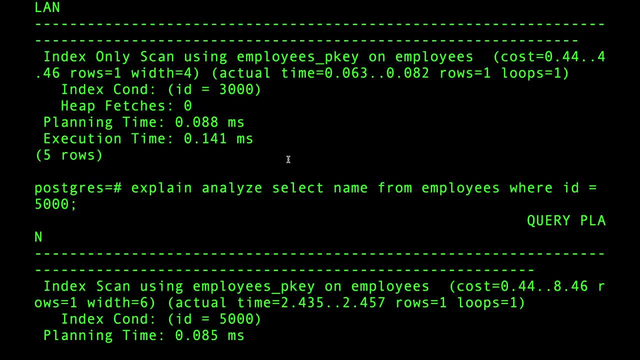 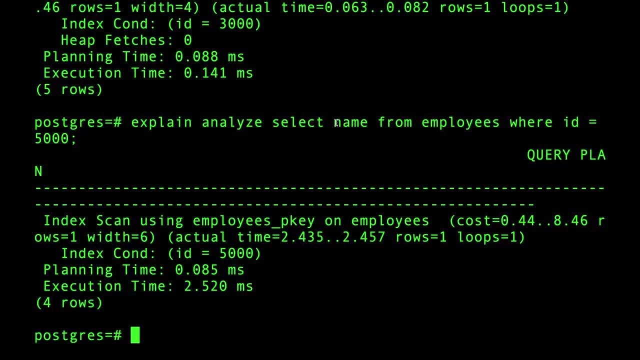 cool, right, It's point. one milliseconds less than a millisecond, which is quite fast. However, when we actually selected the name, which is a column in the table, it is not. the column is not in the index, it is in the table, it's in the. 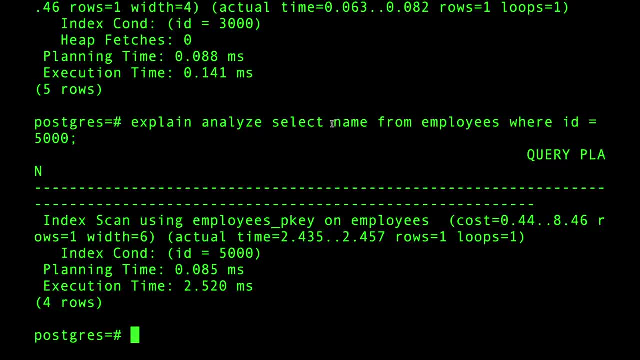 heap. it's in a different data structure, right, And in this case it took us to stinking. two and a half milliseconds, not million, not seconds. two and a half millisecond, which is which is quite fast, but it's still database speak. it's a little. 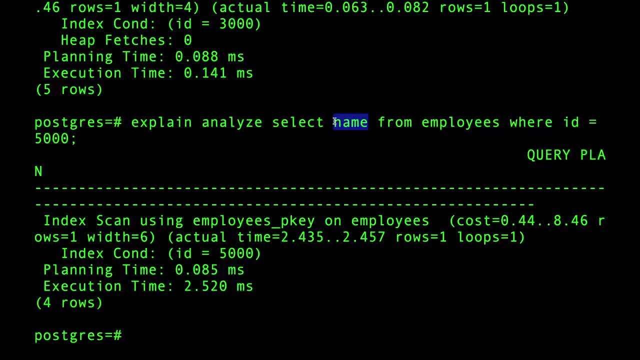 bit slow. This is a slower query And you guys need to understand, when you execute these queries, what it is really mean, because I found the ID in the index but I had to jump into the table row on disk, which is a different structure, by the way. the table 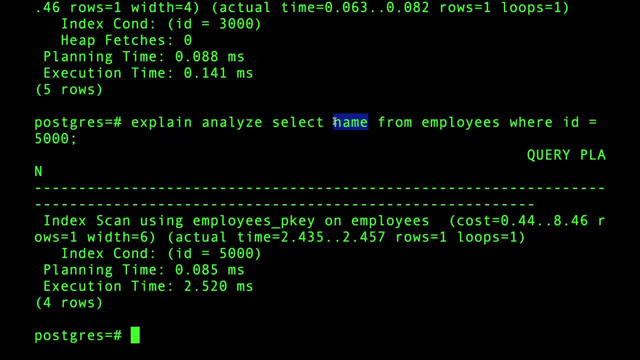 is in a different place than the index. the index is a data structure and the table is a different data structure. right table is actually the heavier thing. we try to avoid going to the table as much as possible because it's there's 11 stinking. 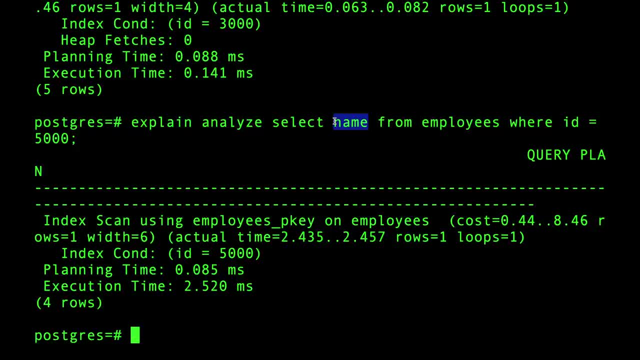 million rows there. So we tried not to touch it as much as well, But sometimes we do. So what we did is we found the ID and then we actually try to go and seek to the disk. I mean, I have an SSD, So there is. 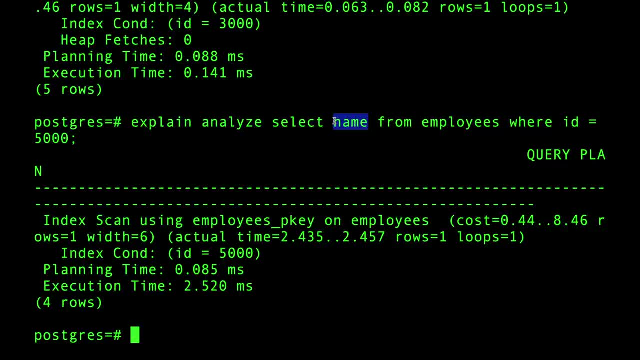 no seek, we go to the page that has this information and we retrieve it from disk. So that's another read from this. So it's a little bit slower. took us two milliseconds And obviously if I execute the same thing again, it's faster. Why? Because caching. 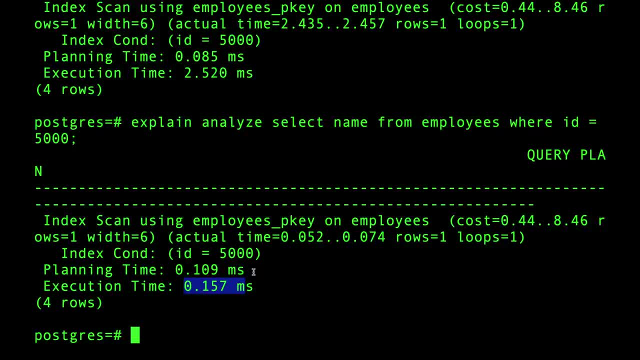 because we cache, things Cache. there's so many cachings going on: SSD caches, the control, SSD caches, the database caches, everyone caches. So God knows what the why's is faster now right, But that's why, because I'm 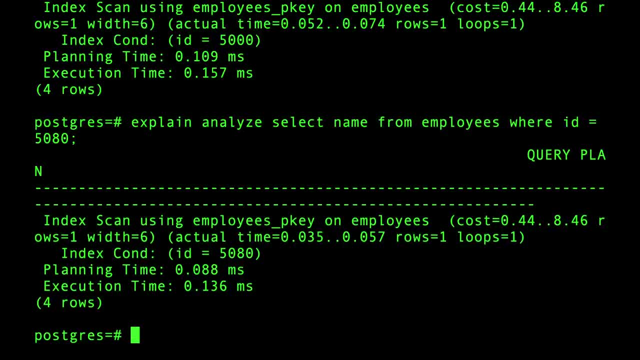 executing the same query. But if I change this to something else I might not get it right, But you get the idea right. Two milliseconds again, Alright. so now I'm gonna spice things a little bit. I'm gonna do explain. 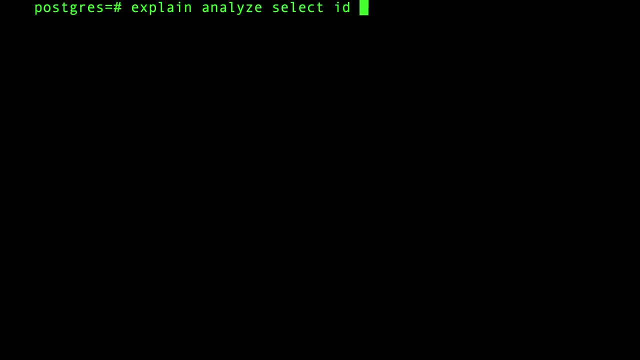 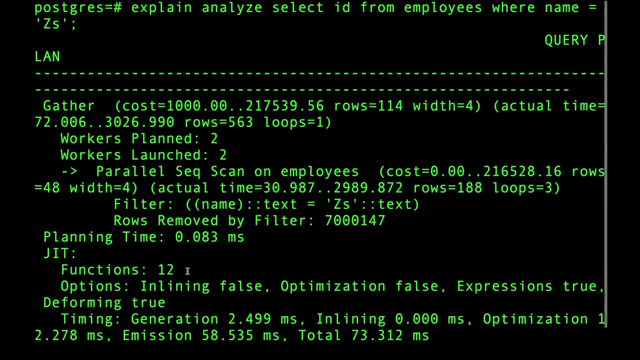 So I'm gonna initialize select ID from employees where name is equal zs. Let's do it. Ooh guys, are you feeling it? You feeling it? right, That was slow, That was that was deeply slow. Why? Because that's what the name column does not have an index And 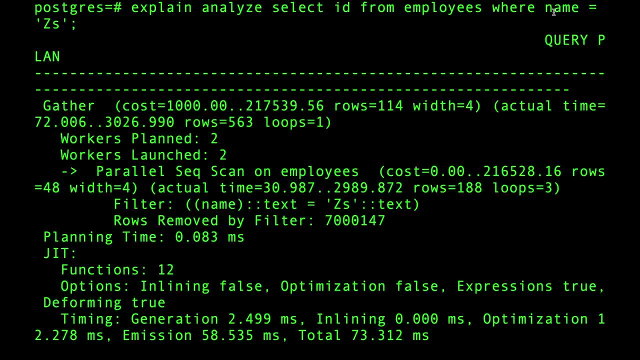 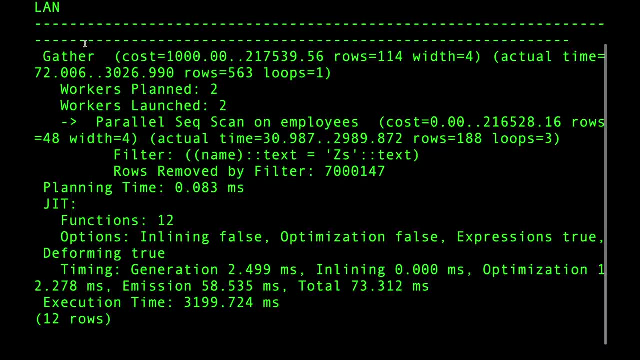 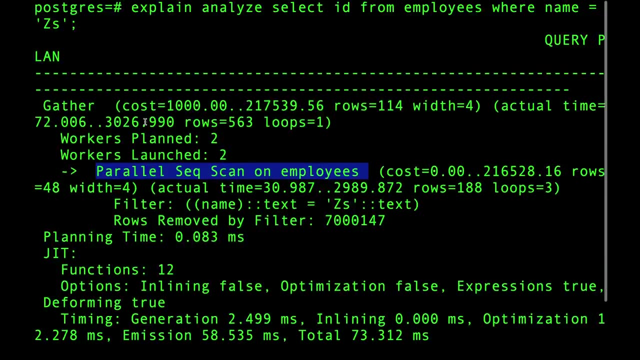 means the only way to actually search through the name, the value zs, is to actually go one by one and do a sequential scan on employees table. that's the worst thing. it's called the full table scan. you want to avoid full table scans as much as possible. however, postgres tries to be a little. 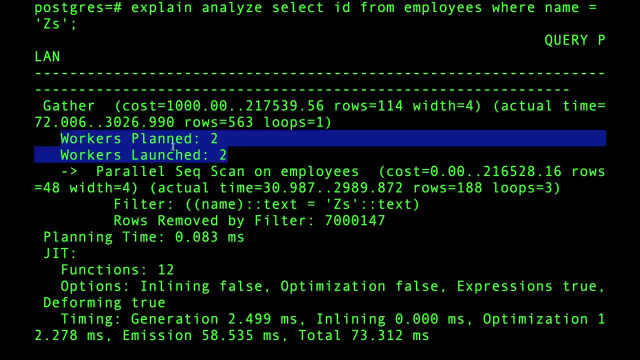 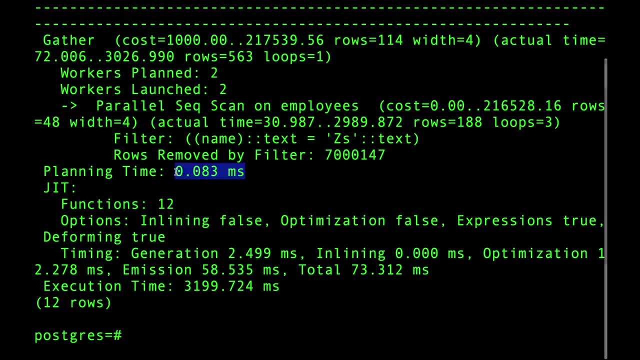 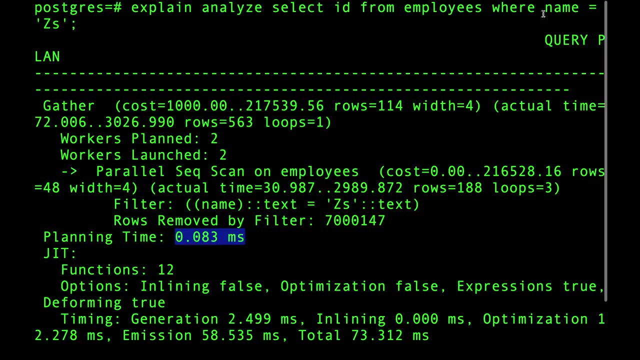 bit smarter by executing multiple threads, worker threads and does. does the sequential scan on parallel, which is still good, right. so the planning took .83 millisecond, which is not much, because well is. does this have? does this column, which is the name, equal this filter? does this have? 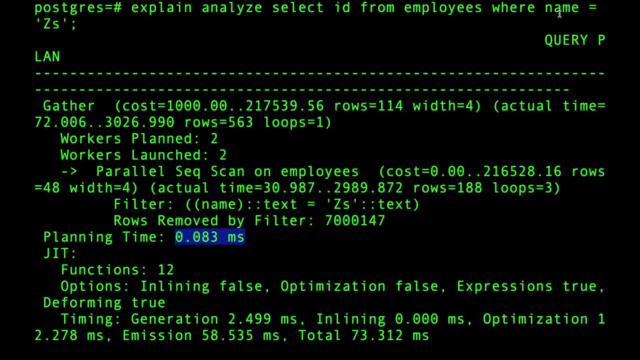 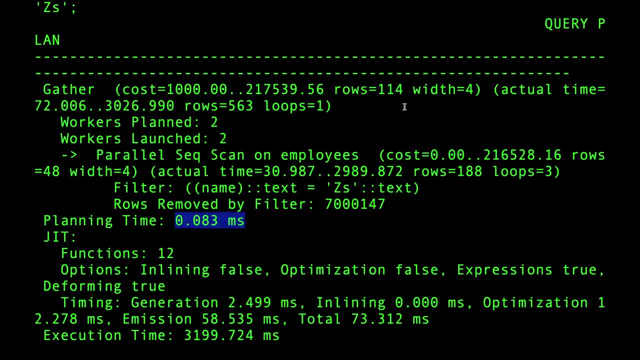 a where clause. does this have an index? nope, it does not have an index. move on full table scan. doesn't have a choice. all right, so it went through and scanned 11 million rows. well, not necessary. well, yeah, it is necessary. i have to scan the whole thing. 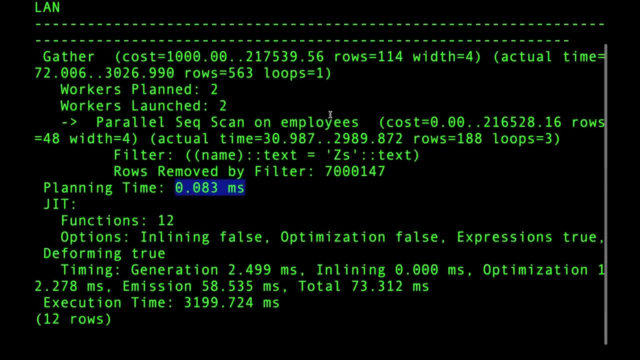 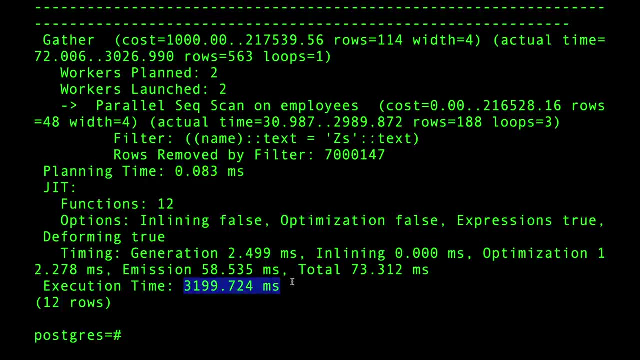 okay, Otherwise, how do you know that? all of them right? You have to check every single one of them, which is the slowest thing. How long did it took? It took three seconds. Yikesy yikesy, that is so slow. 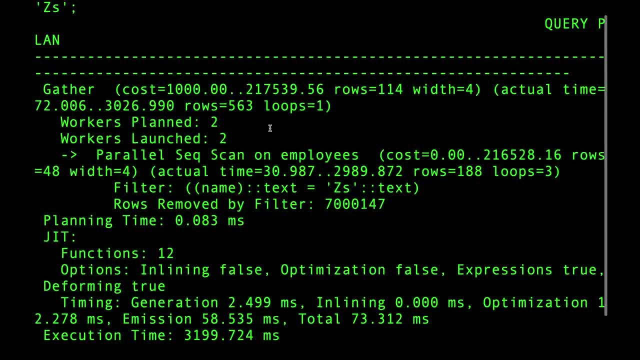 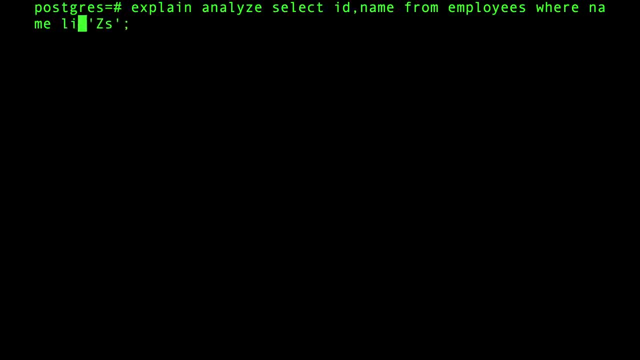 Yeah, so it is pretty slow, guys to do this. Another thing that we notice all the time is- I used to do this all the time without knowing- There's a command in SQL called like. Like, if you don't know, hey, is ZS before and after? 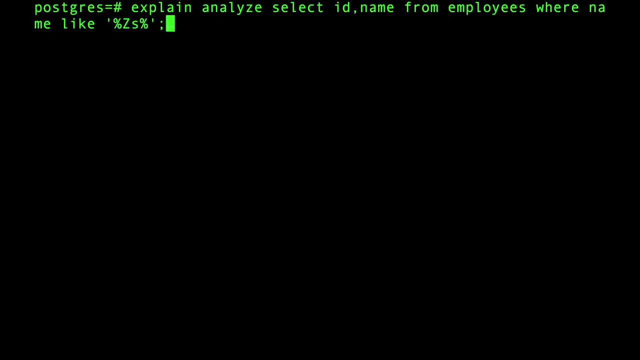 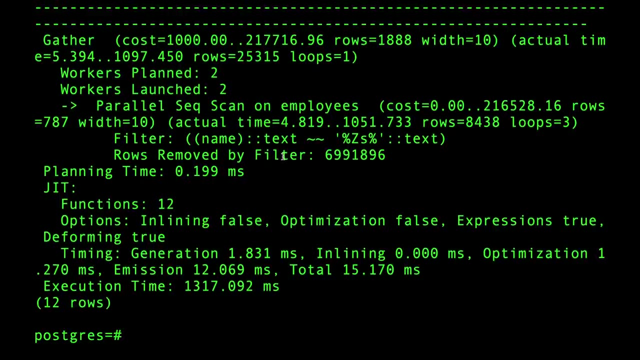 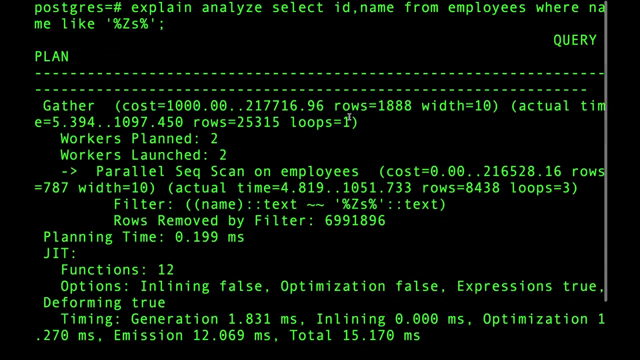 you just add this percentage like This is the worst query. Why? Because it is literally has to go through all the rows and does matching in this case, right, It doesn't really matter because we don't have an index, but I'm gonna show you with an index. 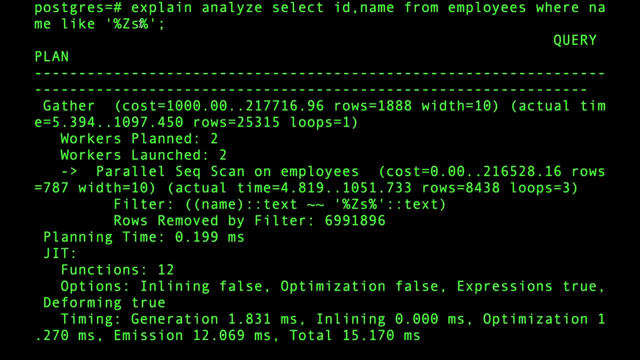 how does it do right? So what this does is it will return all rows that have anything in the beginning, anything at the end, but has to have Z capital as small in the middle. slow, Took 1.1 second to do all that stuff. 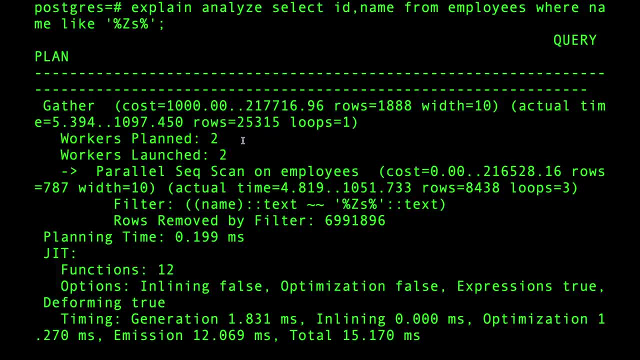 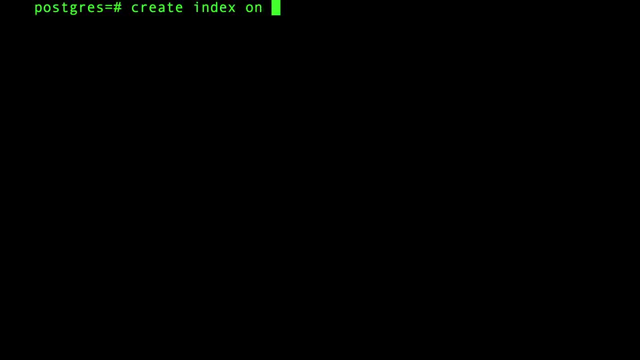 But yeah, so 11 million row, but we had two workers to do the work for us. All right guys, All right guys. so what I wanna do here is actually gonna create an index on- I'm gonna name it- employees. name on employees. 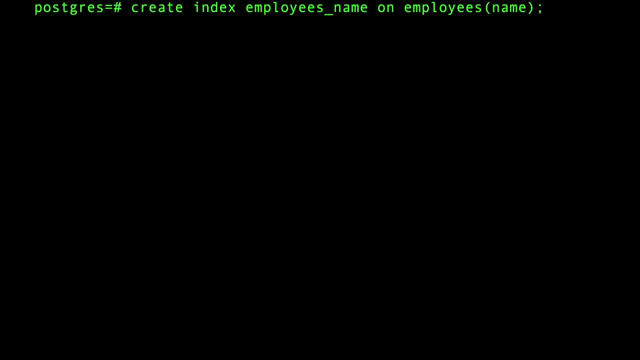 and it is on the name column. So this was going to take some time to create. Why? Because guess what, guys? It is building the B3 bitmap index on top of all the stuff, right? So it has to fetch all the 11 million rows and does all this magic to actually create the fancy index. 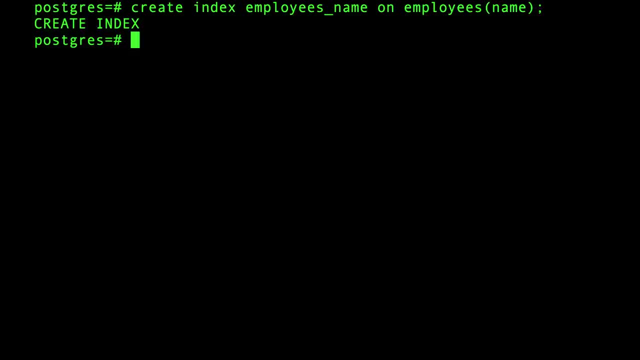 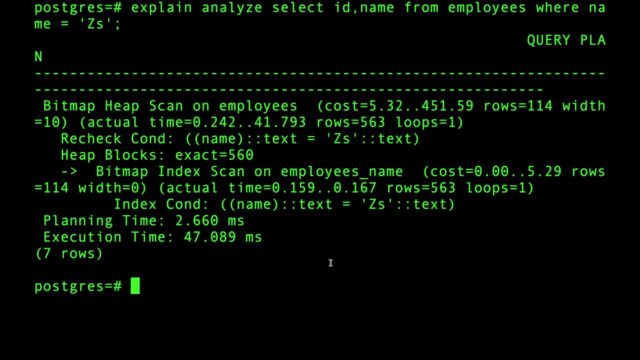 So let's wait for it. All right, guys, we finished creating our index, So now let's try the same query that we have done, just without the like, just directly equal. So now, if I do this query, look how fast it is. Still a little bit slow, 47 millisecond, but damn, that was quick. 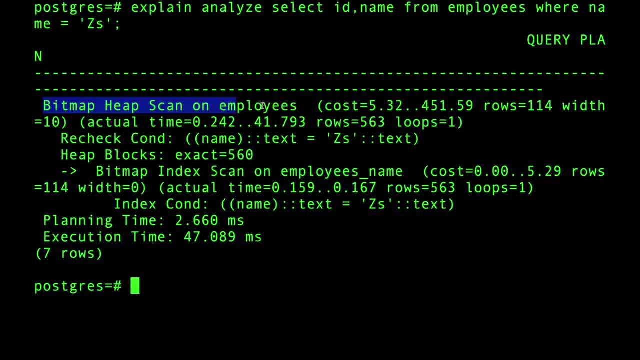 Why? Because now we're doing a bitmap heap scan on employees, Right? So we're using the actual bitmap index scan on employees name, So we're actually scanning the employees name index that we created, And this is way faster because we have fewer rows. 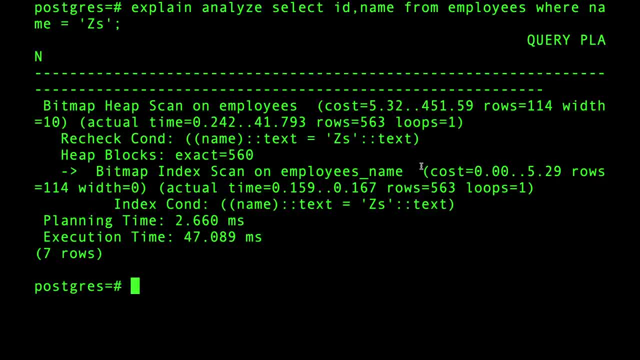 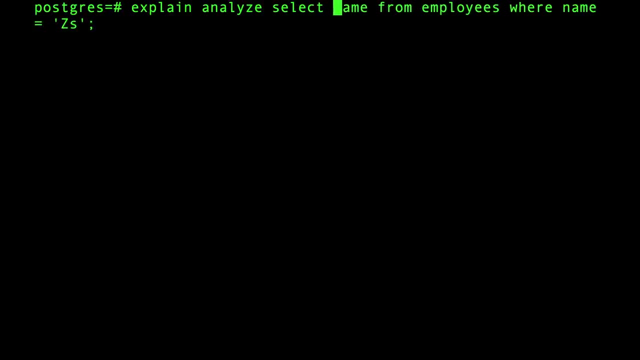 to work with And we're going to actually jump between few rows until we find exactly what we're looking for, Right, And obviously, guys, the same thing applies where if you only pull the name which is already in this index is going to be faster than pulling the. 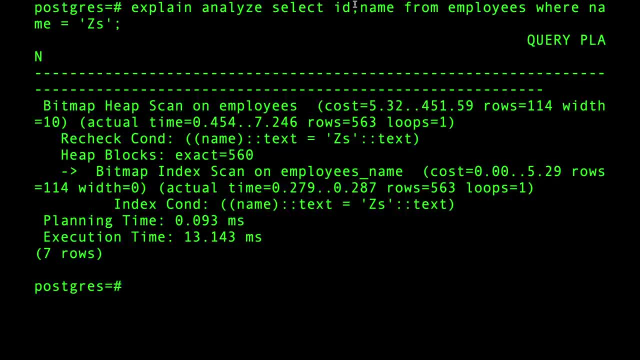 ID and the name. I'm not quite sure about this. Maybe this actually doesn't hit the heap because the index, the primary key- I know this is in MySQL. I'm not sure about Postgres, but the primary key is usually stored with every single index in other databases, Right? So the 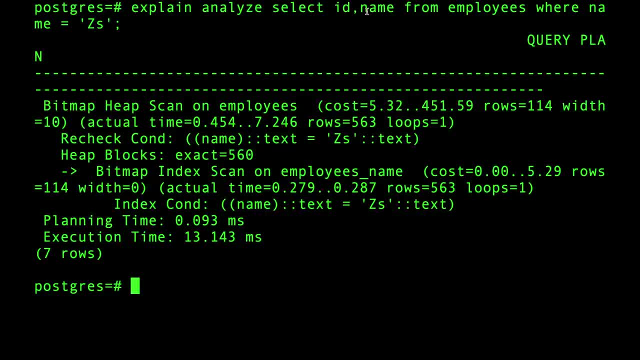 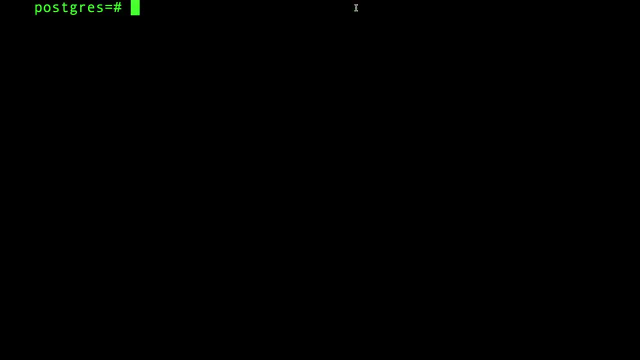 primary key will be stored. So pulling the primary key from the name index will be fast, because it's it's right there, Right with it. So, however, if you're, if you have more than other tables, then we had to go to the table structure and that will be a little bit slow. All right guys. So what will? 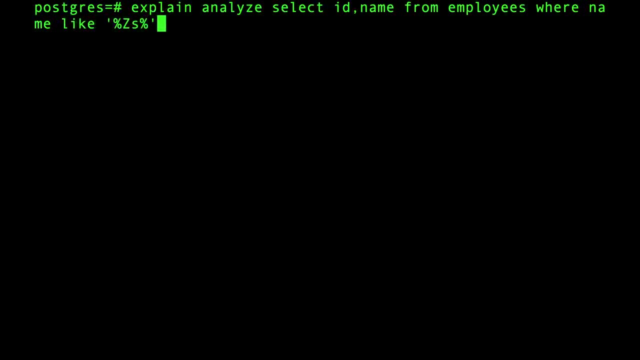 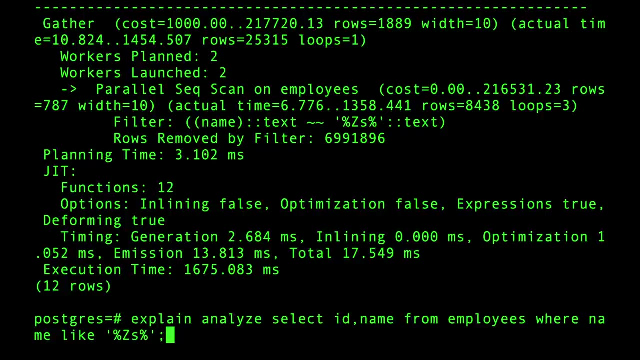 happen if I add, like here: What do you think will happen? Back to the slow query, back to the exact same slow query guys. Why, Let's clear this again. Let's do it, Let's do something else So we don't have way ahead. the. 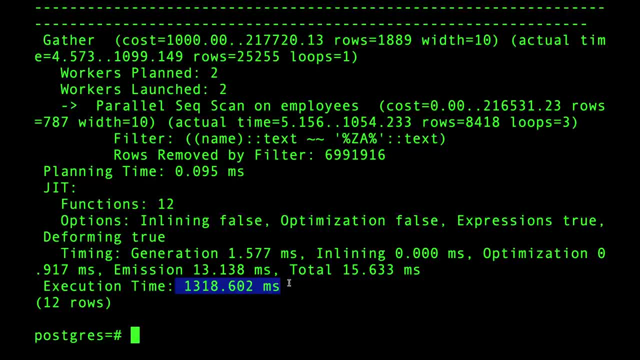 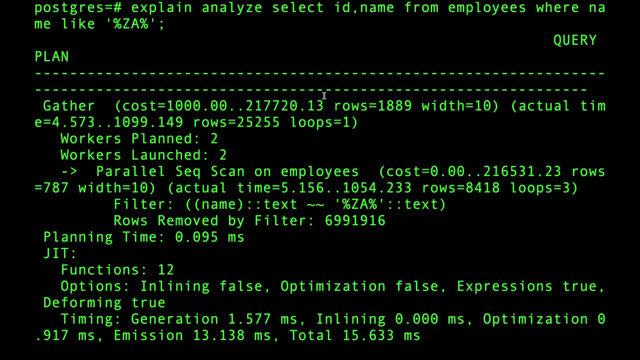 cache. Yes, back to the same slow query. Why? Because we could not scan the index. Why This is? this is a lot of people make this mistake. Yeah, the name column has an index, But what you did is you're not actually asking for a for literal value, You're asking for an expression. 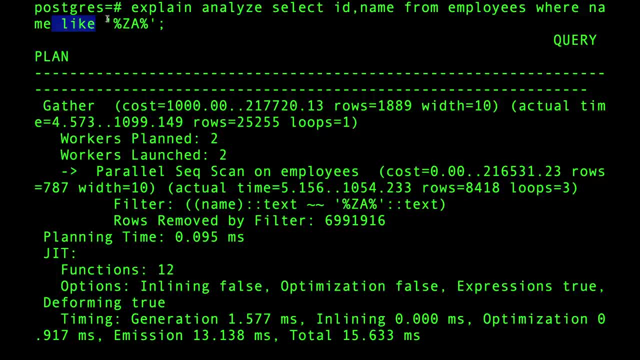 And there is no index that will satisfy this expression, Because we cannot search the index on this, on this expression, because there is not a single value. So the planner quickly detects this, says okay planning time. we check this then then, Oh sorry, the filter sucks And that's why. 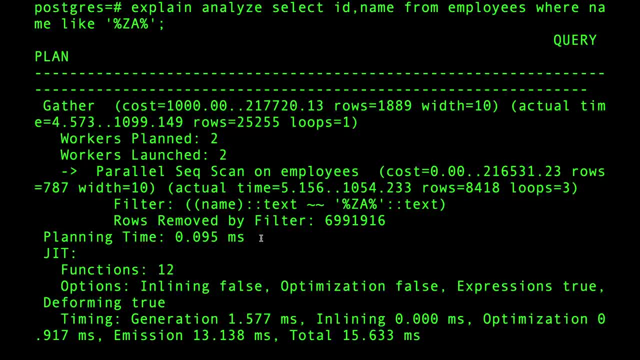 you have to do, explain on your queries and see why are they actually slow? Because of this, because, look at this, we did a parallel sequential scan, again parallel. not all databases do parallel scanning, by the way, but that, postgres though, we did, we had to do it. we had to go to the 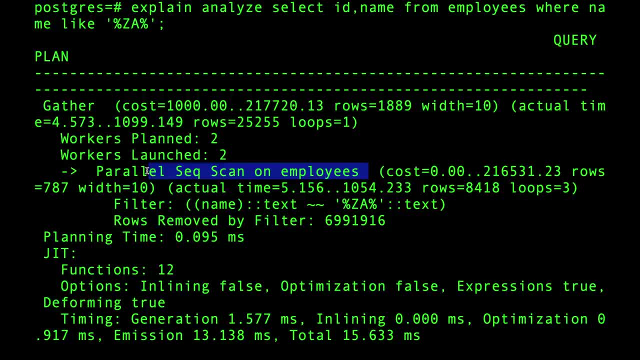 stinking table and scan my 11 million rows. if I have a billion rows, it's gonna be even slower than that. So, yeah, going through all that stuff- And I'm going to explain all this number in other videos, because I don't want to make this video longer than that- I'm going to make an advanced. 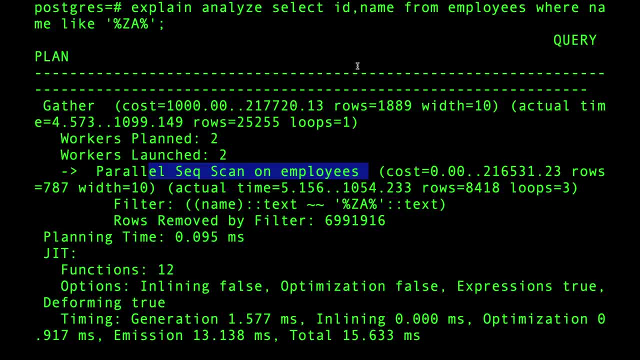 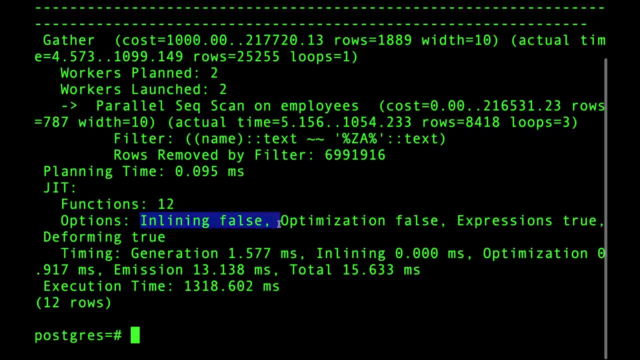 video discussing these actual numbers or what do they mean, all that stuff. But But yeah, we did a little scan on employees guys, look at that, It's so slow. we couldn't do inlining, we couldn't do any optimizations- And this is an expression, obviously. so that's we had. we had to do all that. 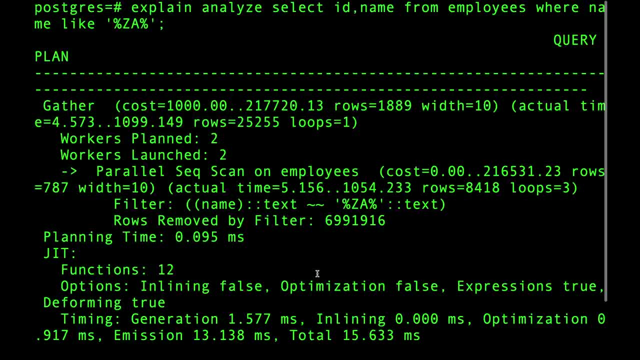 stuff. So we took a hit. we took a hit despite us having an index, guys, despite x having an index. So, guys, that's very quickly indexing. in a nutshell, in a very, very quick video I wanted to explain of that. Yeah, having an index does not mean that. 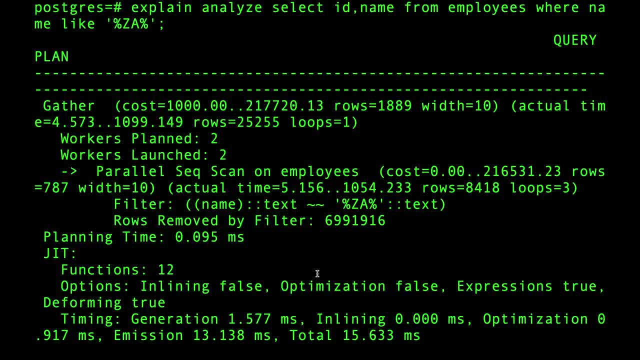 the database will always use it. it's gonna plan and, according to the planner, will decide to use the index or not. It's up to you, as as the engineer who's executing queries against the database, to actually give hints to the database to actually use the index or not. right, This is a bad query. 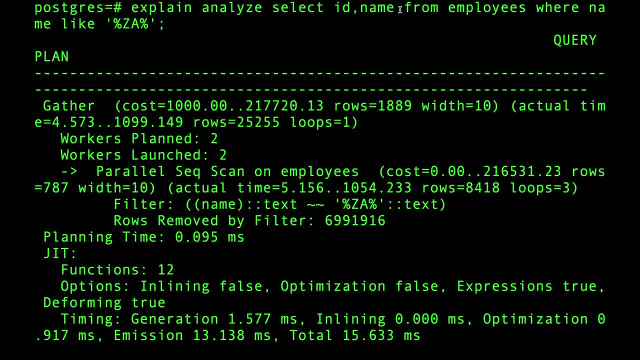 in general, select star is a bad query in general. Why? Because, if you, because if you think about the cost to go to the actual disk and pull all the information, that is expensive, right, Really really depends on how much, like, let's say, you have. 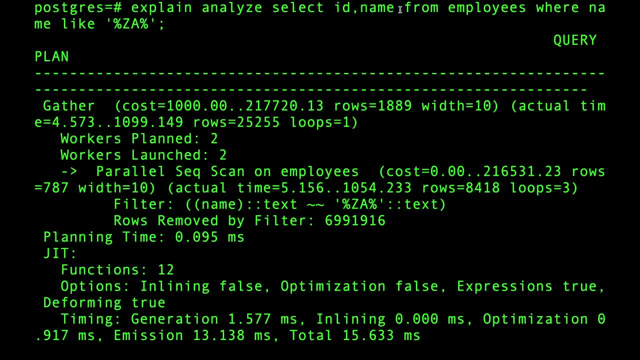 a blob or column on the field on the table that is expensive to pull up. So if you don't need it, don't ask for it, right, And only ask for things that absolutely there. And if you can ask for things that are in the index, right. I'm going to talk about that in another video. we're just like: 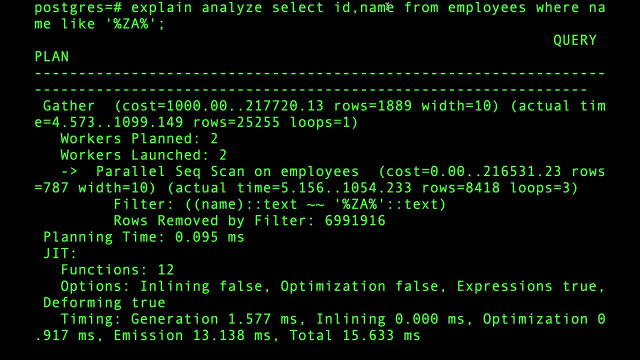 multi column index where you can add other columns in the index that you're about to create. this is called inlining, where, where, as I search my beautiful index, my neat, efficient index, I want the name, for example. right, that's bad example. 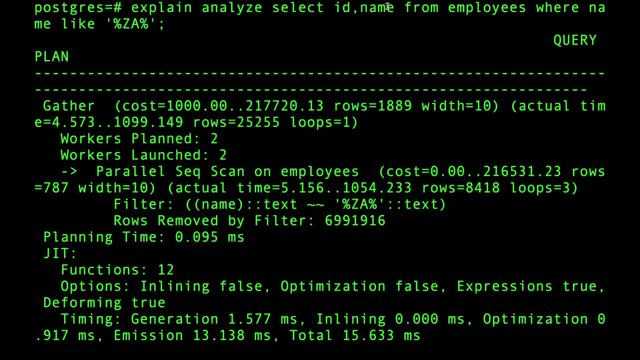 but I want the name. I'm searching for the ID and I own the name. oh, the name is right there. it's just literally sitting in my index, So I just pull it and retrieve it to the user I don't have. 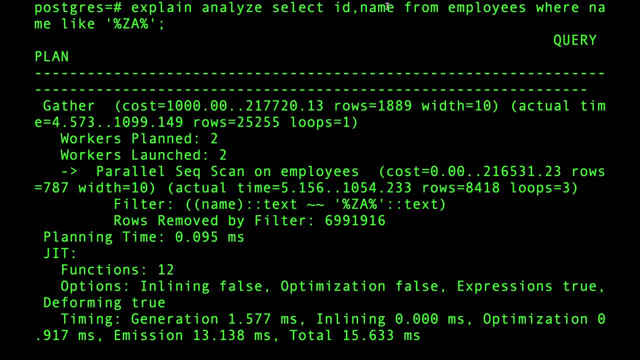 to go back on disk and find the location, seek in disk if that's a mechanical drive, or pull the name in case of SSD. guys. Alright, guys, that's it for me today. I'm gonna see you in the next one.